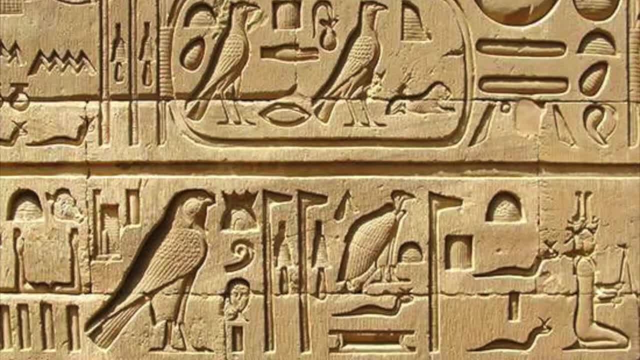 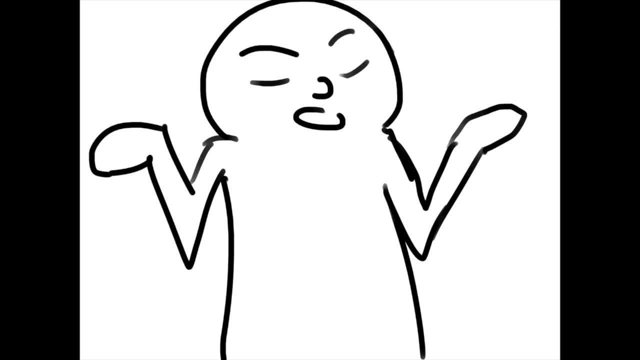 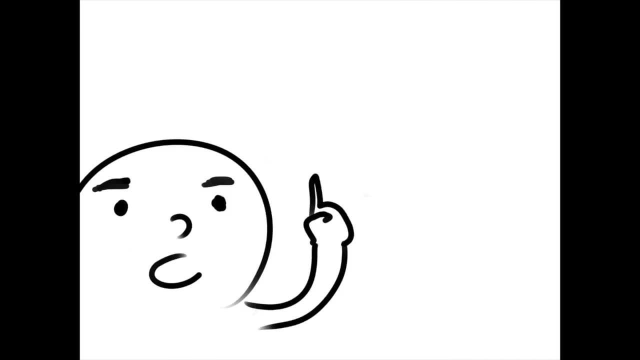 vague definition, slow video or one of these. Impedance is dumb And it's stupid And it's stupid And it's dumb. But that's okay, It's alright, Because I'm about to explain all this shit right now. So what is impedance? Well, if you looked it up into any one of the dumb articles, 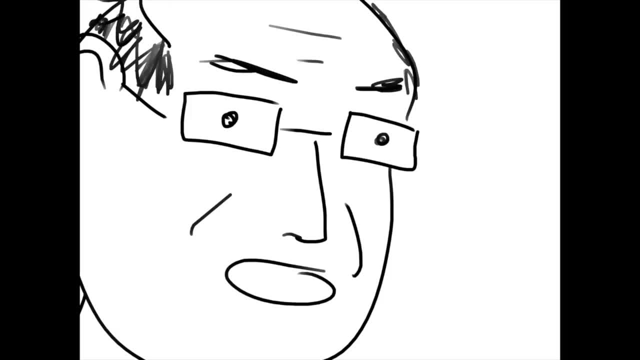 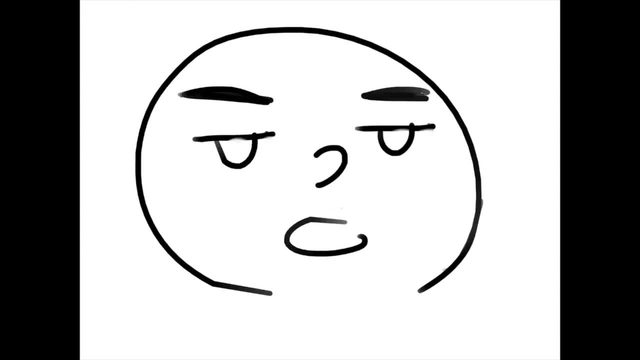 I've been talking about. I can guarantee you'll find something along the lines of impedance. Impedance is the extension of the definition of resistance to alternating currents. Okay, so what this means is that impedance includes two things: Resistance to AC. 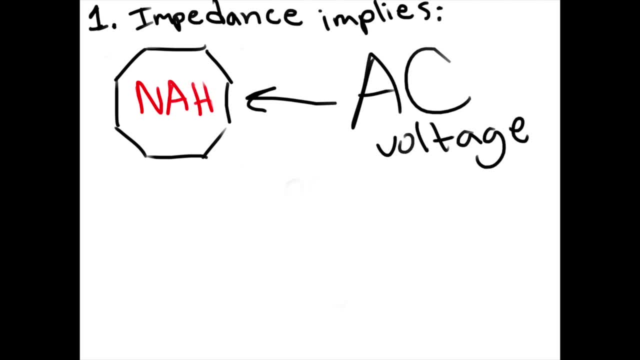 which stands for alternating currents, And the resistance being the opposition of the electric current that causes heat, And the second one being reactance. This is the measure of the opposition itself. What the fuck are you talking about? Well, here, look, Impedance is basically. 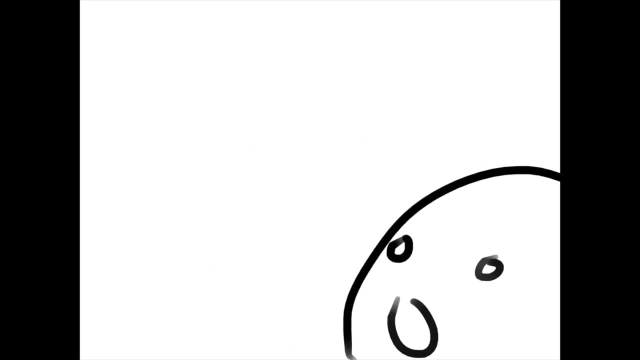 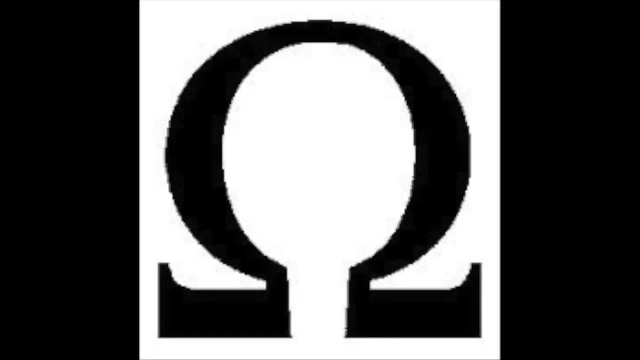 the resistance to electricity. Oh Okay, Well, Whatever. But hey, If you don't pay any attention to these things called ohms, you might blow up your goddamn speakers. Yes, this is necessary to pay attention to. You're an engineer. 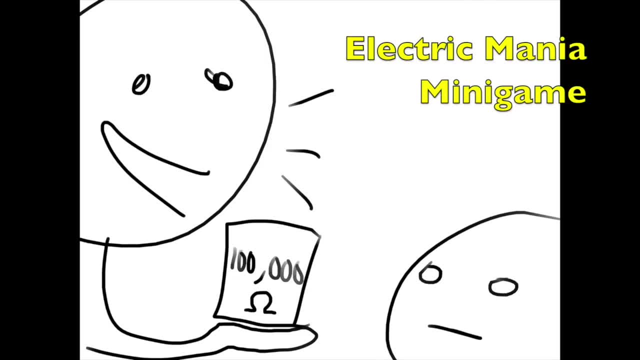 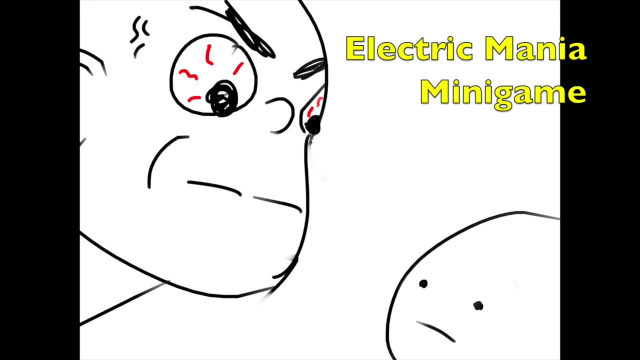 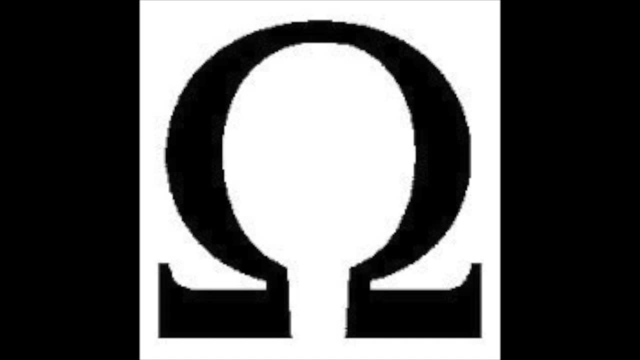 not a visitor to Electric Mania. Guess the voltage: Winter Prize: A hundred and de действ请 Hall. No, Its too low, Okay. so what are these ohm things we're talking about now? An ohm derives from ohms law, Ohm's. 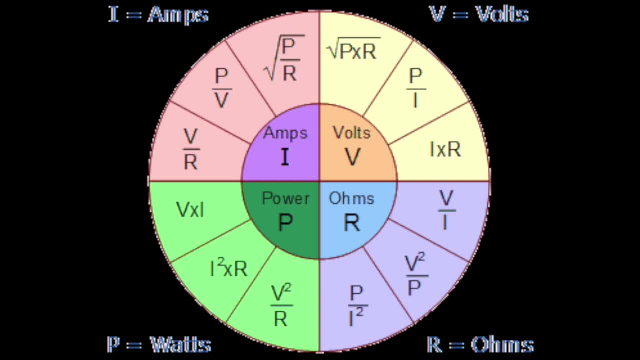 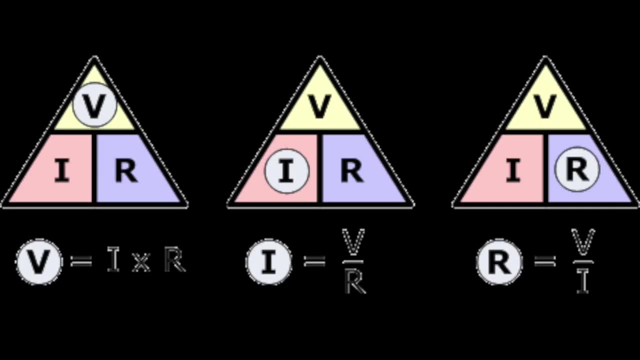 Ohm's law states that the current through a conductor between two points is directly proportional to the voltage across the two points. Proportionality, aka the resistance, is determined by the usual mathematical equation that describes this relationship, which is: V equals IR. 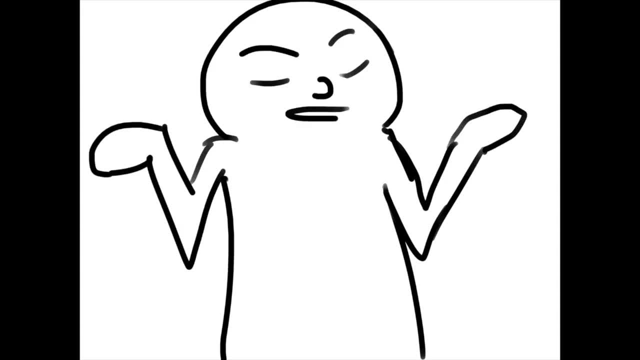 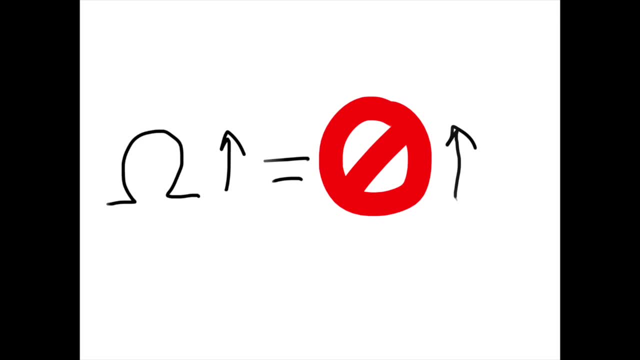 See, doesn't this look familiar? We all know what V equals IR is. I don't get it. Okay, well, to put it in English: basically, ohms are units of resistance. The more ohms you have, the more resistance there is. 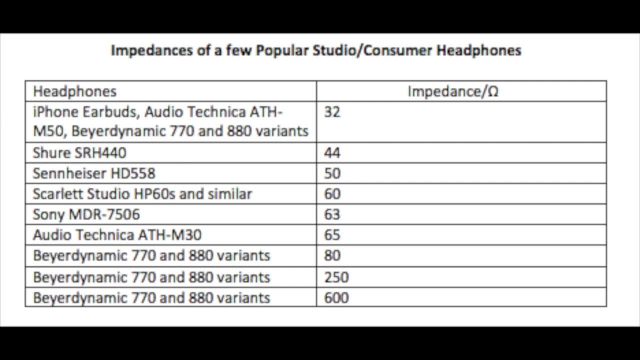 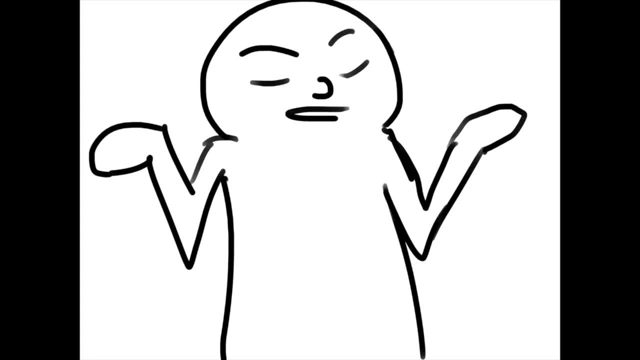 So these ohms are generally what you're gonna be seeing on, like your headphones and stuff like that. Let's put it in a real life situation: You buy a headset but the thing has 50 ohms. There's no way in hell your computer's garbage sound card that came with your motherboard. 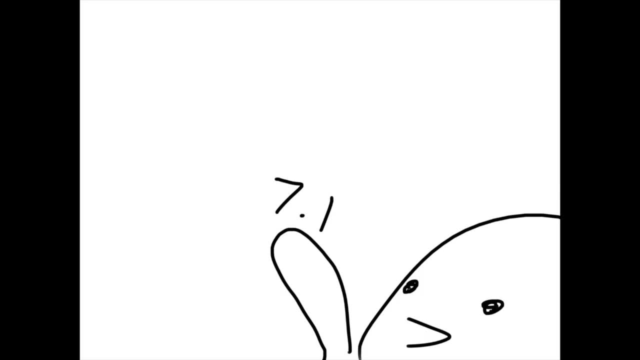 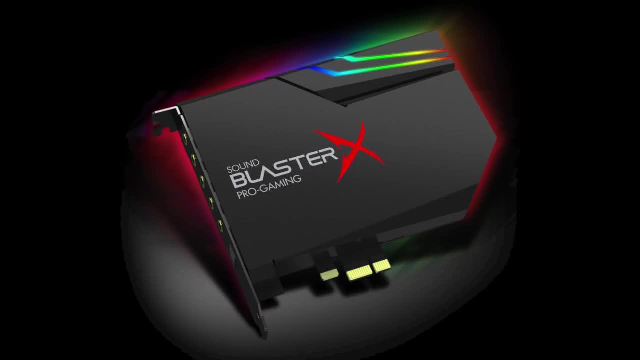 is gonna be able to power that thing without it sounding like a donkey's ass. But my computer has 7.1 surround sound support. Doesn't matter, We're talking about the ohms here. To power that thing you're gonna need a sound card that has the proper voltage to support.